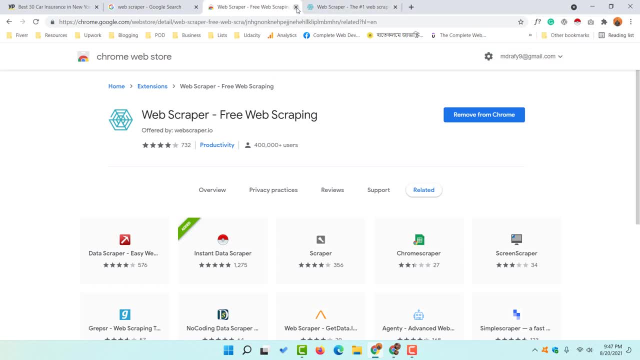 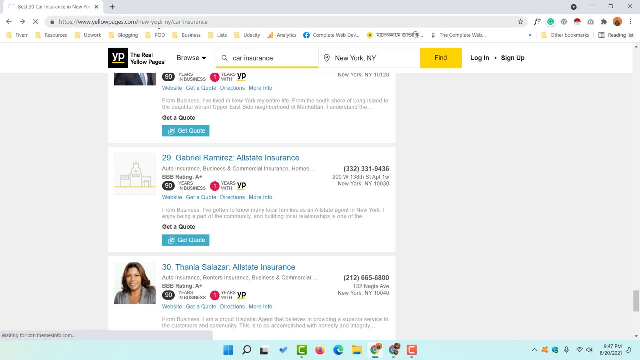 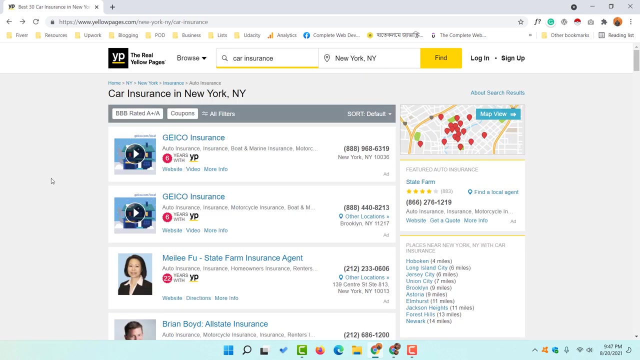 free web scraping has been added to Chrome, So now we are all set with the tool installation. Now it's time to reload our search result page on yellow page or whatever directory that you'd love to scrape data from. Alright, so here we go Now. after reloading the page, simply you have to click on the right button of your mouse And then you are going to find this inspect option, Or you can use a shortcut key, which is control plus shift plus i, But I'd love to 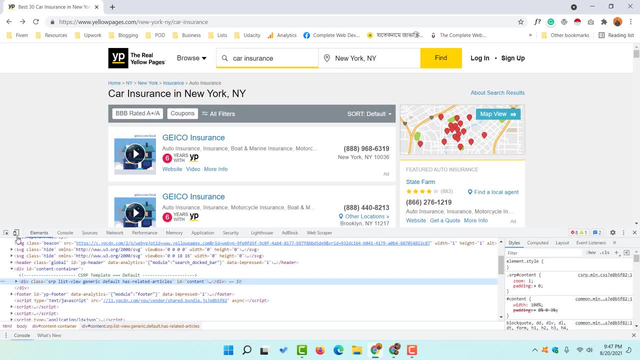 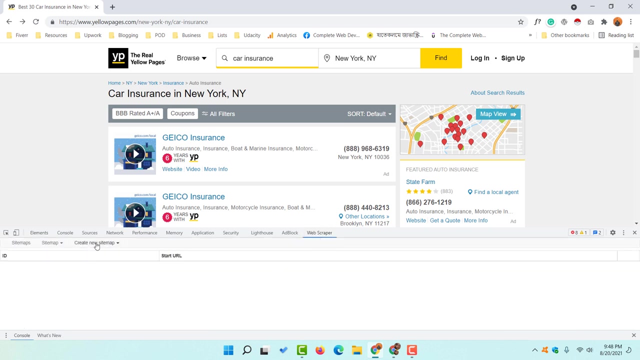 click here on this inspect button so that we'll get this console tab or this console information into your browser, right? So after coming up here, you are going to notice this option: web scraper. if you have installed the extension already on your Chrome browser, you will notice this button or option, So let's click on it. After that you have to click on create new sitemap And then we are going to click on create sitemap And then we are. 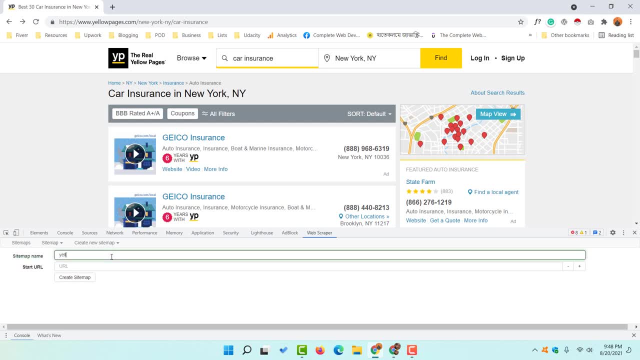 going to check out the to give a name to the sitemap. so let's say i'm going to type out yellow page extraction and the url start url is going to be this url, copy and paste it and then click on create sitemap. after that we have to add a new selector for this root sitemap. so let's click on add new selector. 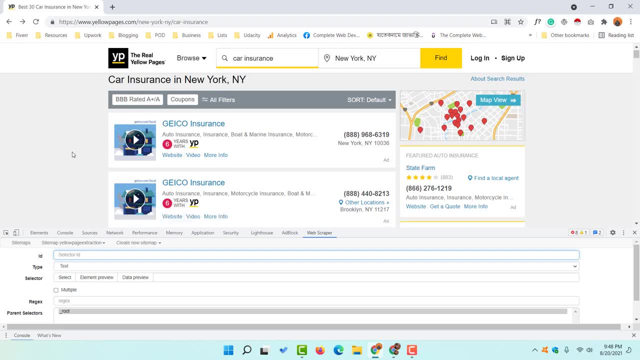 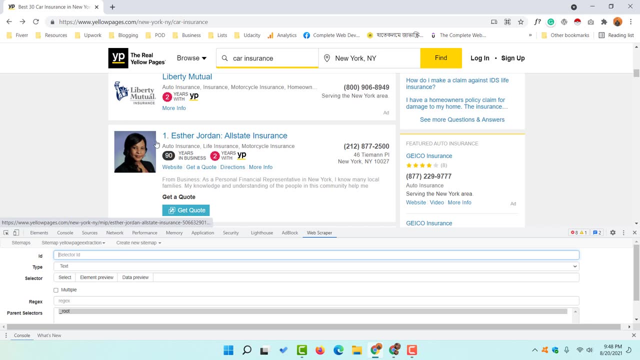 and then we are going to select. on the first stage we are going to select all of the business listings page or these links. let's say this is the first link for the first, business, professionals information. then we have got. this is the second link for the second, business or personal. 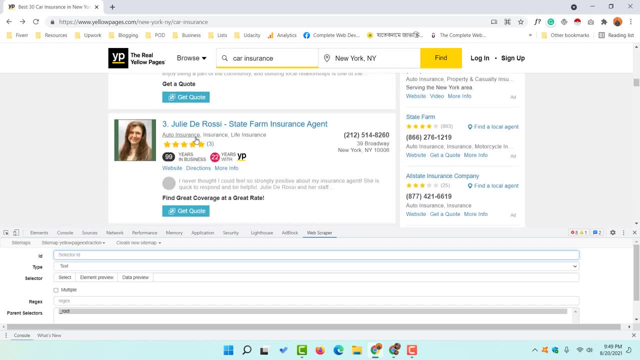 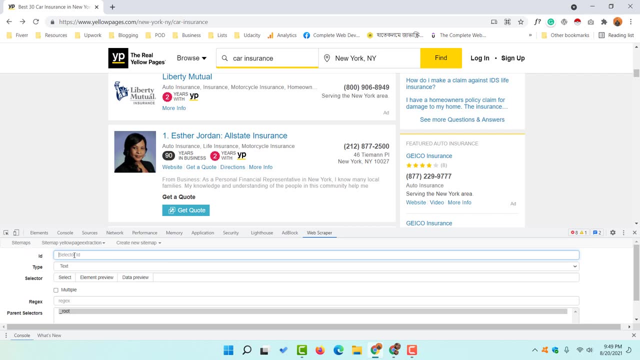 person's information right, and so on. we have got third, fourth, etc. so now what we have to do? we have to click here, and then we have to provide a id name which is, let's say, i'd love to give it as links, and then we have to change the type from text to link, and then we are going to select. 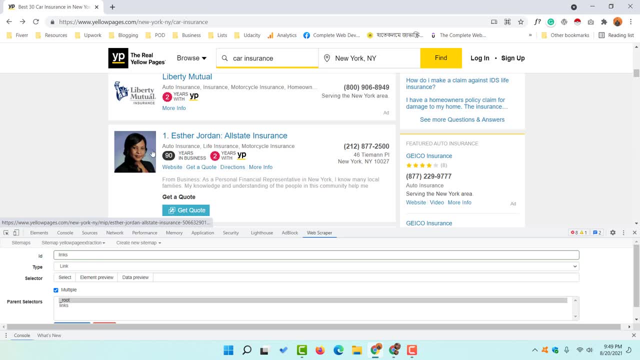 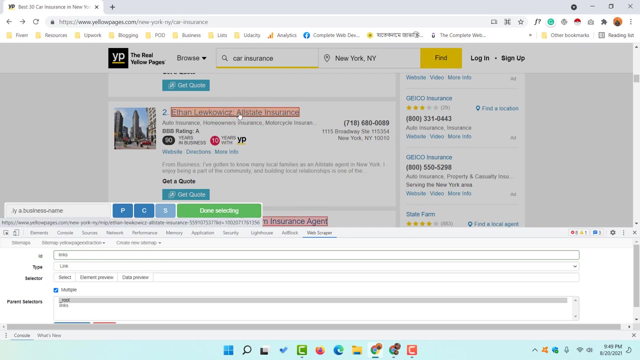 multiple. as we are going to select multiple links from this page, let's say so. we are going to click on select now. after that we are going to click here and just take a look. the name of this person has been selected. after that, go a little bit down, click on the second listing and if you just click, 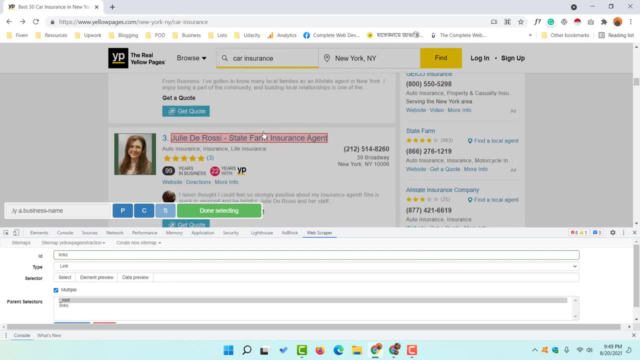 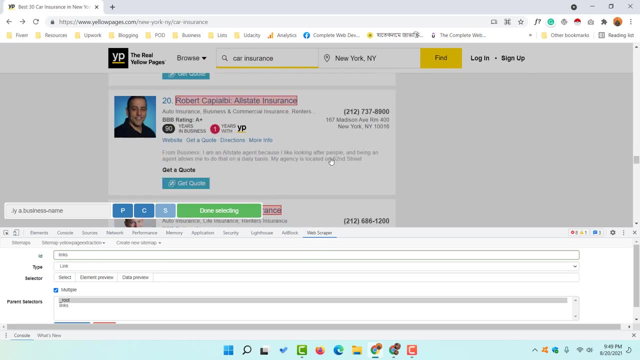 on the second listing, you will notice that rest of the listings has already been selected automatically and the tool worked for us, right? so if i take you to the bottom of the page, you are going to notice that we have selected all these 30 profiles already, right? 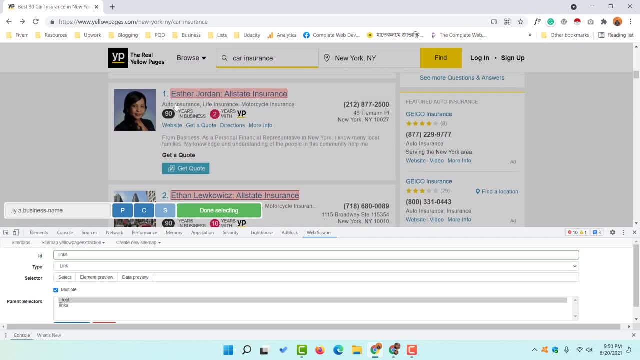 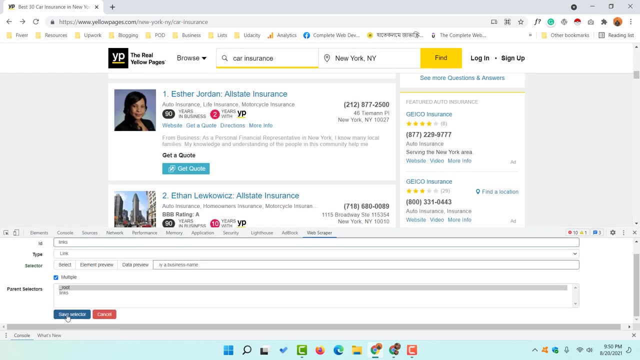 so now let's go to the top of the page. so after selecting these listings, we have to click on done selecting button right here and then go a little bit down. you will find this option: save selector. let's click on save selector. we are done with creating our very first. 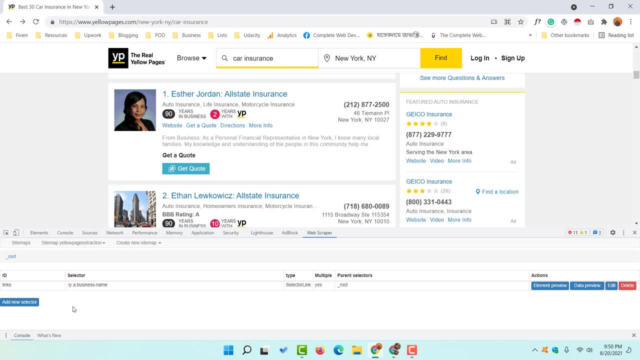 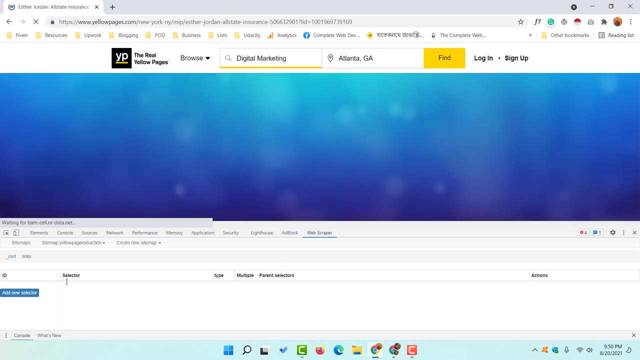 selector. now what we have to do? we have to go inside the selector, because now we are going to collect information from this business listing inside this business listing, so let's click on it. after that we are going to click here as well, on this id. and now we are inside the first selector. 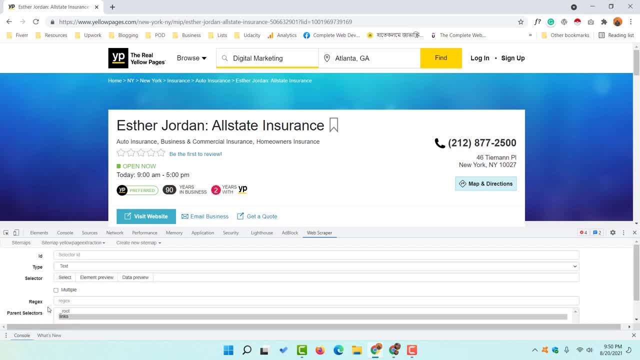 now what we have to do. we have to click on add new selector button right here. after that, we are going to select the business name so that the name or the id name is going to be, let's say, business name or let's just put name here, because i have noticed some of these profiles. 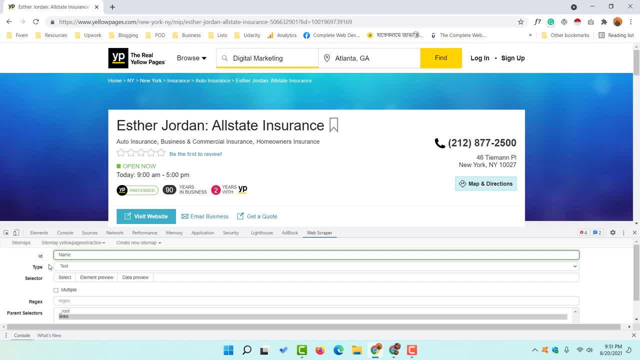 are personal profiles. some of these profiles are business profiles as well. after that we can keep the type to text. then let's click on select and then we are going to select this business name. just take a look, it's just selected. now let's click on done selecting. after that we are going to 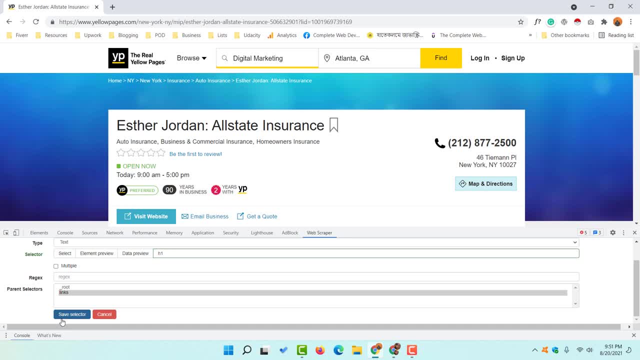 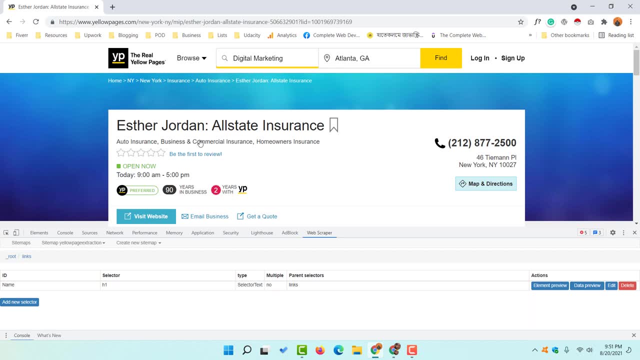 the bottom of the page or this option, and then click on save selector. so we have selected our uh, so we have just selected this parameter for taking our business name. now it's time to select another selector for um, this phone number, address and all of this information. 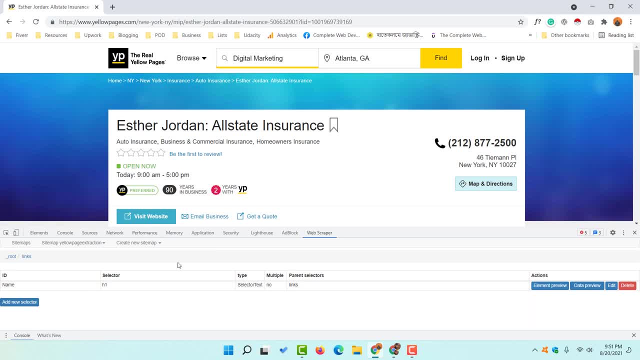 so these are basically. these two are basically the repetitive task of the first one, but we have to make a little change here on website and email address collection. so let's just click on it and then we are going to collect, let's say phone number, and then click on. 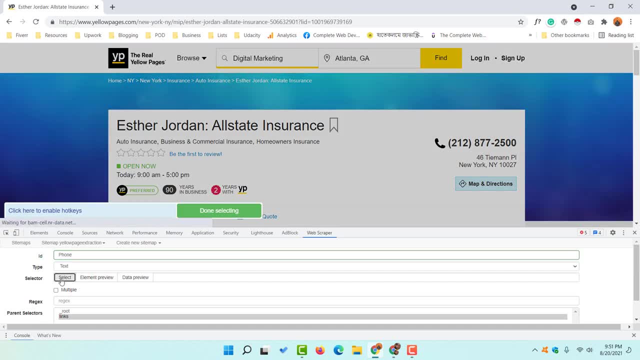 keep it as text and then click on select. after that we are going to click here so that the phone number will be selected. let's click on done selecting and then we are going to click on save selector. after that we are going to click on add new selector again. after that we are going to 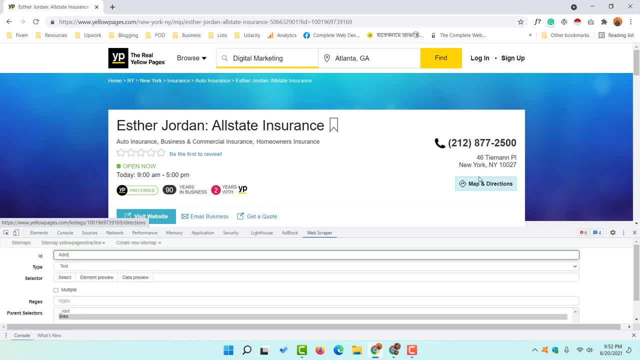 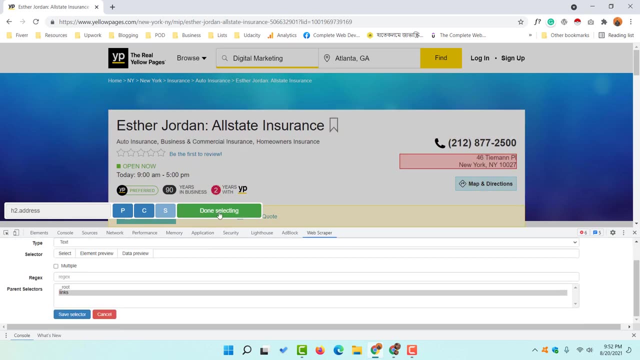 give it a name, let's say address. after that keep it as text. click on select. then we are going to select both of these lines. so click here so that both lines has been selected. now let's go, or sorry, we have to click on this. done selecting. 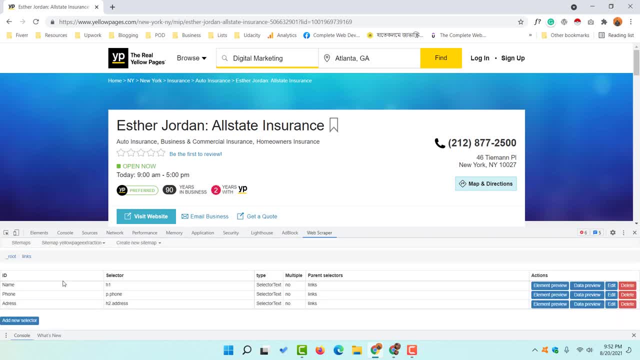 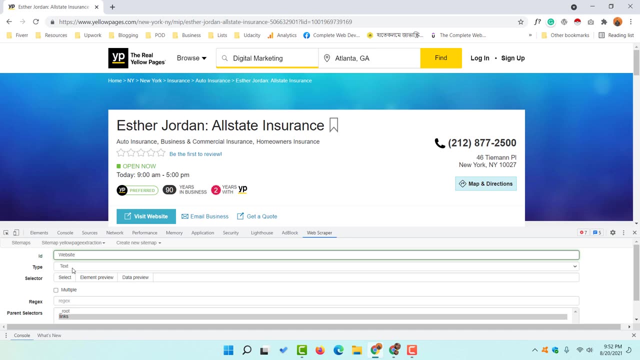 and then we have to click on save selector. okay, so we are done with all of these phone number, address and business name selection. it's time to select our website. so let's click on add new selector. after that we are going to give it a name. let's say website. after that we have to change the type. 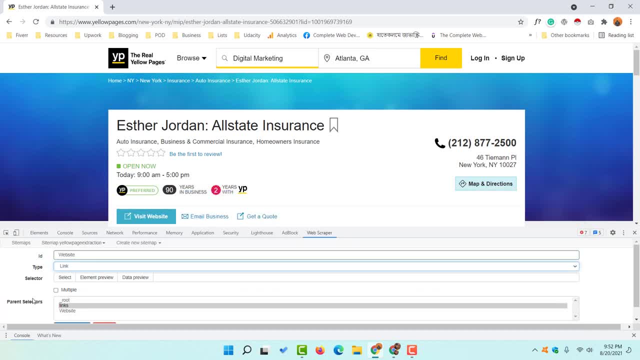 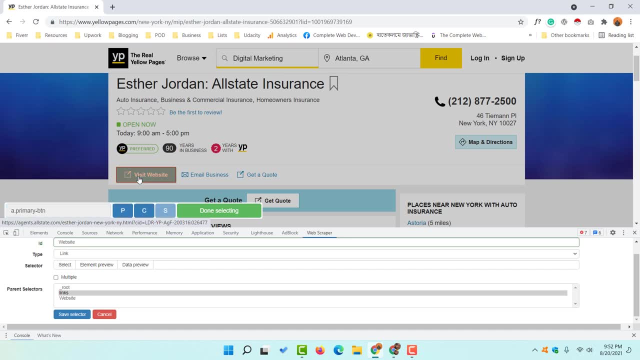 from text to link and then we are going to click on select and after that we have to click on this visit website button right here and we are going to click on this see, then click on done. selecting. click on save selector. now let's do the same for. 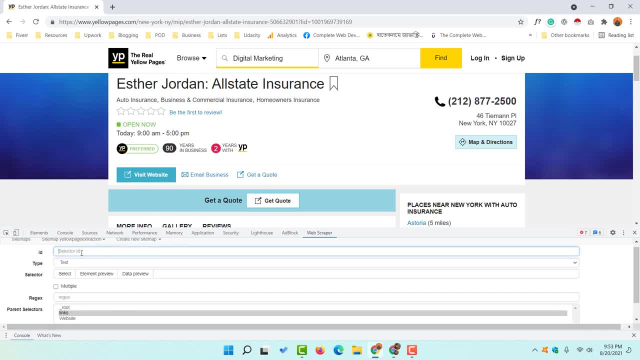 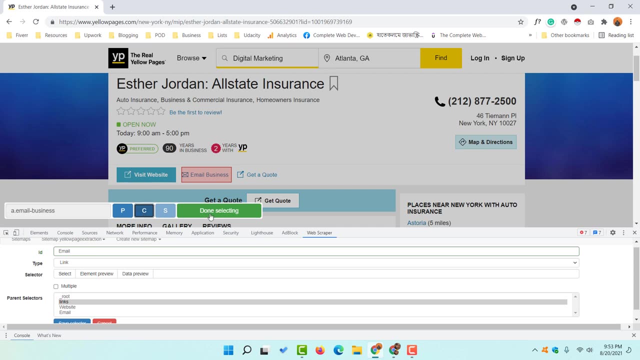 the email address, let's click on add new selector. after that we are going to type out email and then change the type from text to link. after that let's click on select. then we are going to click on email business on see. we are going to click on done selecting. then click on this save selector. all right, so. 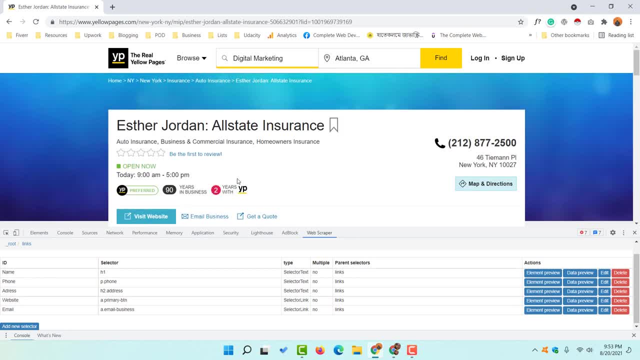 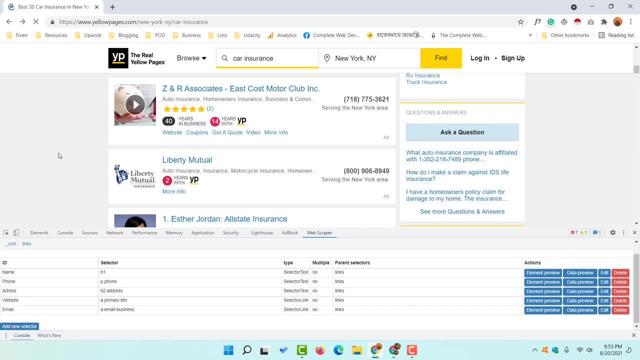 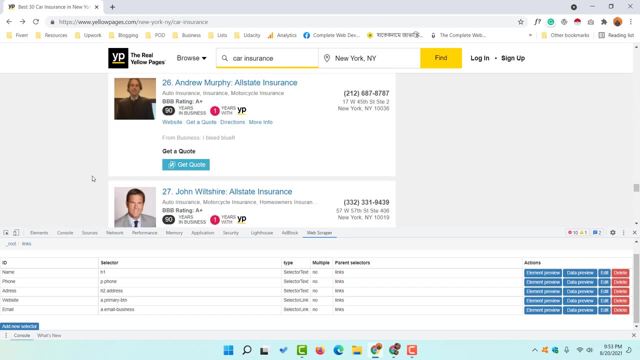 we are done with this page information selection. now let's go back to the previous page by clicking here. so if we run this scraper now, it is going to collect information from all of these 30 results from this page only, but we have got few more pages appearing here, so now it's time to select. 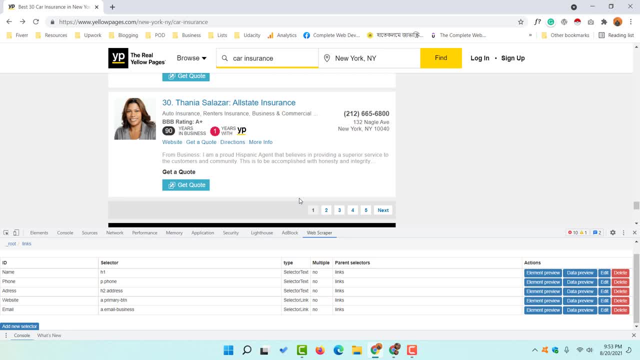 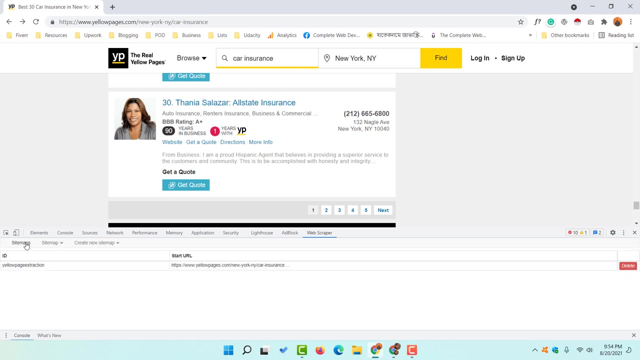 these pages as well, so that our tool will go to this page and then get information, as they are going to collect from the first page listings. to make this happen, we have to go up, and then we'll notice this option: sitemaps. let's click on sitemaps. after that, we are going to click here inside this. 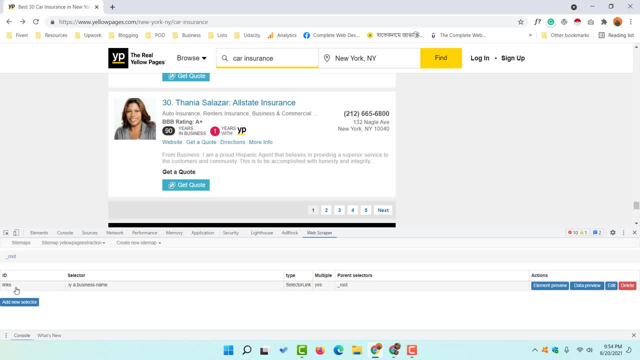 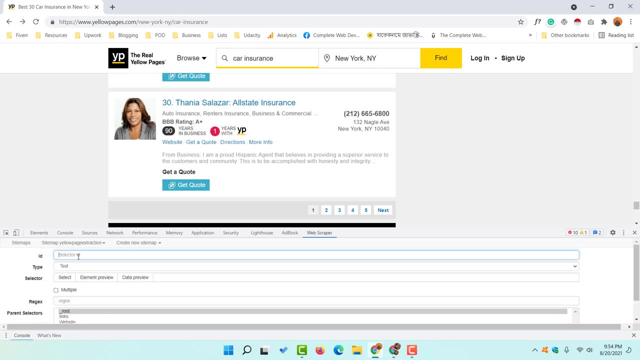 let's say sitemap. we are going to find our first link, sitemap. then we are going to click on this add new selector button right here, and then we are going to add a new id. let's say, these are pages. so i'm going to type out: 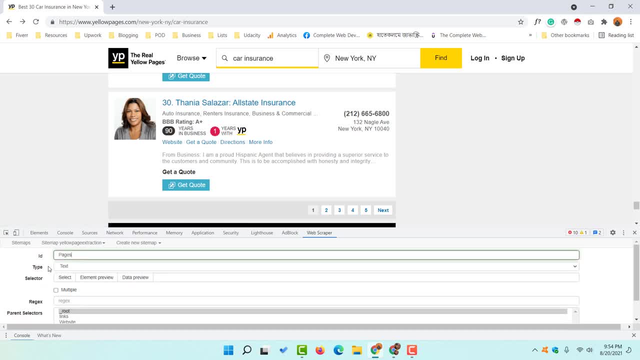 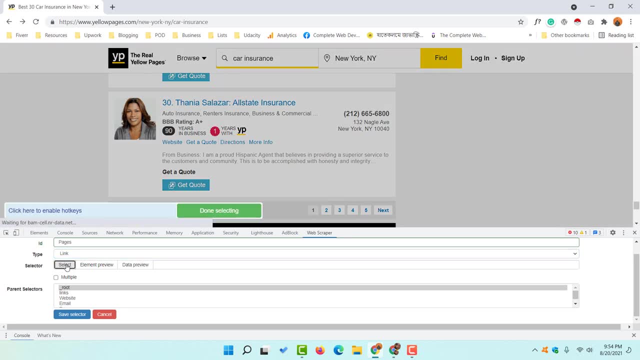 let's say pages. after that we are going to change the type from text to link and then we are going to click on select, and this should be multiple. as you can see, we have got two, three, four, five next. so we're going to click on multiple. then let's click on select. 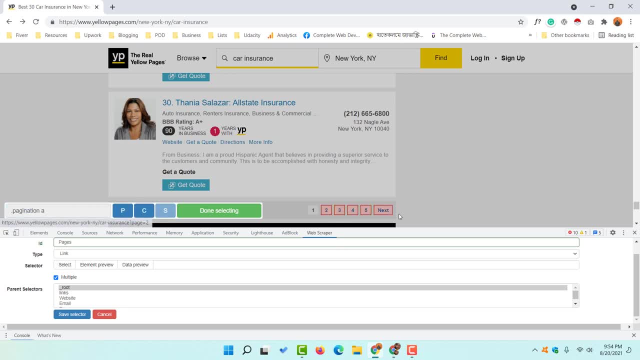 and after that i'm going to click on two, three and just take a look. it automatically selected two, three, four, five and then it is going to go. if there are the six, seven, eight, nine pages, it is going to go on these pages as well as the next also selected. now let's click on save selector. 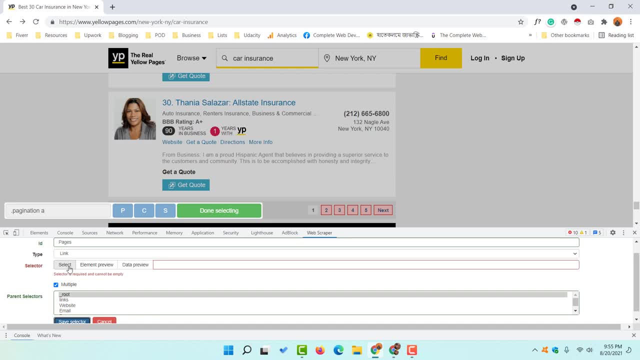 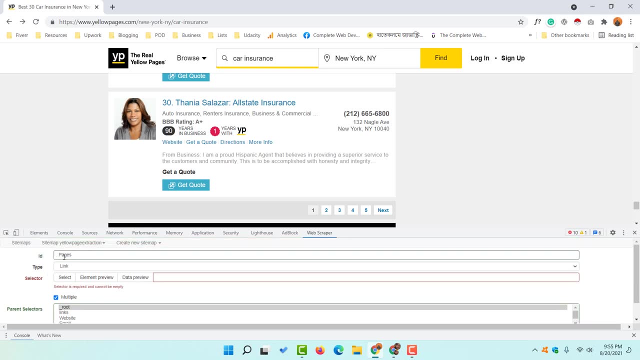 button right here. okay, so i've missed something, so let me click on select again. yeah, okay, so let's do this part again. so again, i have provided the id here. pages type is link. now it's time to select it multiple and then let's click on select. after that we are going to click here on two, three and 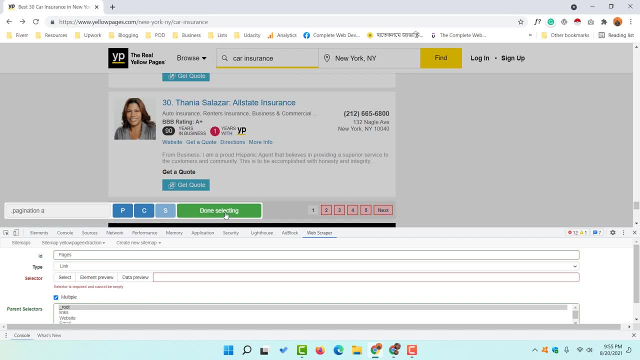 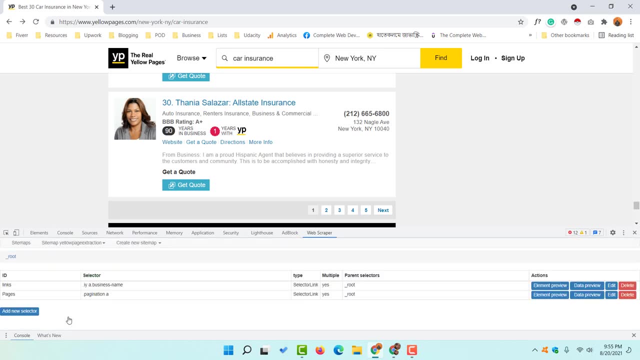 it is going to be selected, all of these pages. now let's click on done selecting. okay, so i actually missed this part. so let's click on done selecting and then we are going to click on save selector. now one more thing we have to do here. we have to go here on the first selectors edit option. 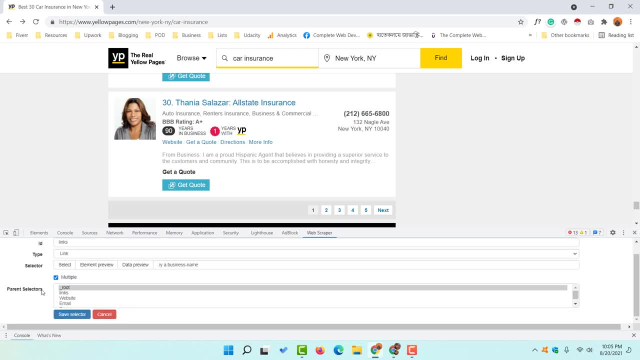 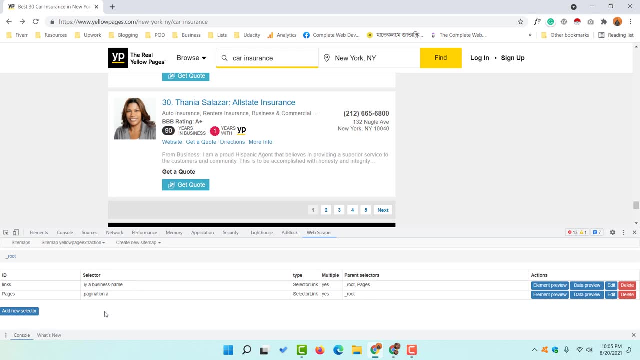 and then from here we have to select, as you can see, parent selectors. we have to select and the pages. now let's click on save selector. after that, if we go here and click on this option and click on selector graph, we are going to see the graph of what we have done so far. so just 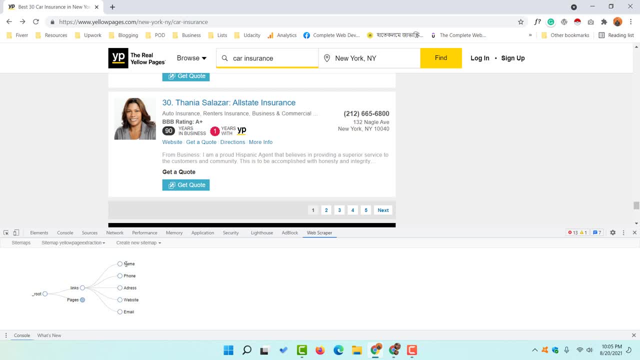 take a look from links. we are going to find all the pages. just take a look: name, phone address, website and email. these are the points we have selected. now, if i click on pages, it is going to show us inside from pages. it is going to visit each of the links. 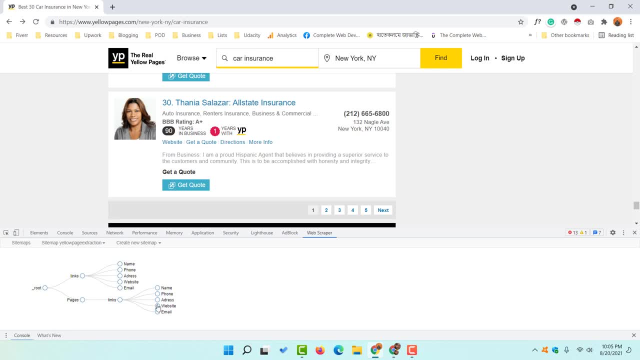 and then it is going to get all the information from here. so our repetitive task has been settled properly. now what we have to do? we have to go here, then click on script button right here and then make sure you have settled a large number here. let's say, 2000 is the basic, but the more gap you 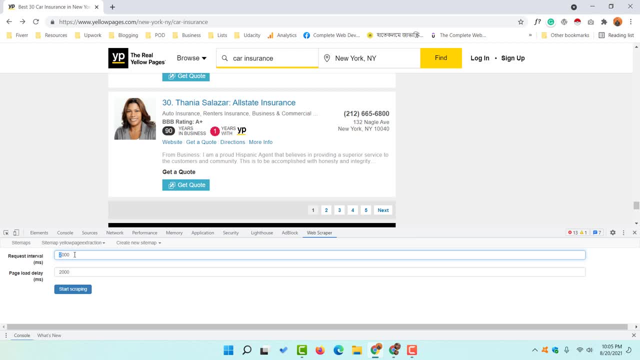 are giving on the intervals, the better it is going to work on the website, because most of these business directories or website has some limitations of accessing their website from a views a user each day. so after visiting, let's say, 10, 15 pages or more than that or whatever their limit is, after visiting these pages they 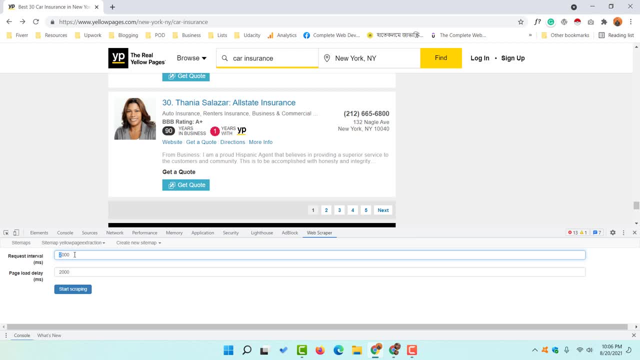 are going to send you a restrict message, restriction message- or they are going to make the tool stop. so in this case, if you provide, let's say, 7 000, your chances will be less to get stopped faster. so in this case, as this is a tutorial purpose, so i'm going to select 2000 millisecond. it is going to work perfectly. 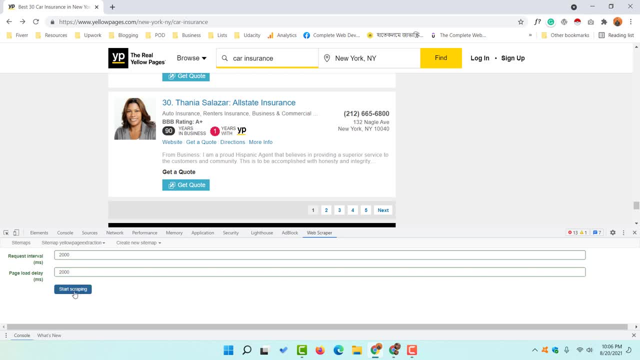 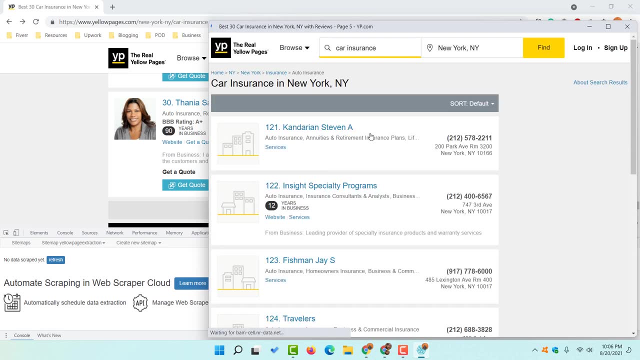 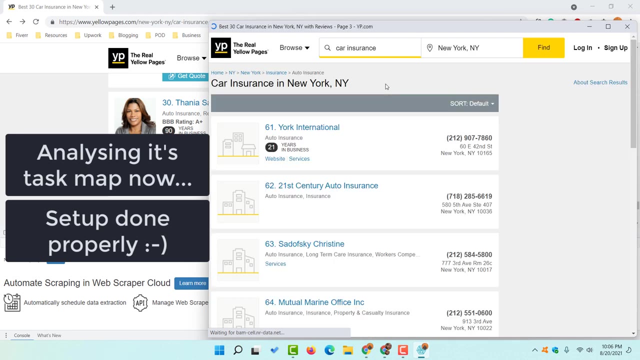 fine for this tutorial purpose. so in this case, i'm going to click on start scraping and it is going to start visiting each of these pages automatically and just take a look. it is working here and okay, let's just wait. just take a look. it's already been visiting the 61th listing, 31th and 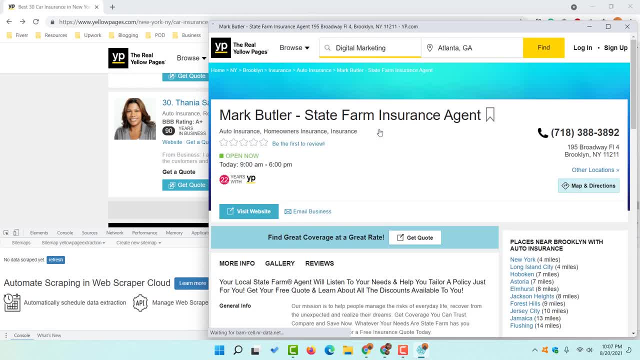 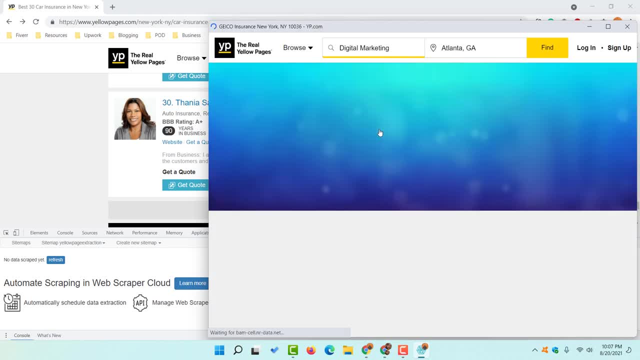 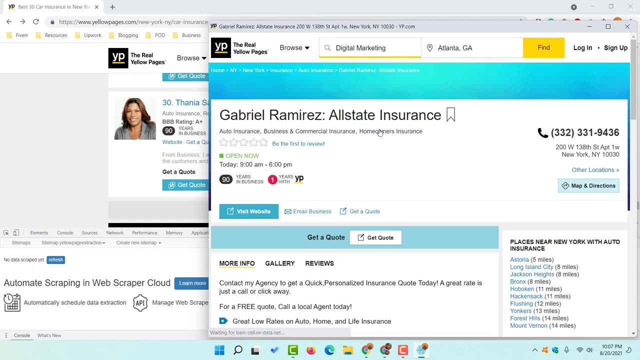 here it is visiting the first page and, yeah, now it is going to visit each of the persons or businesses profiles. it is going to collect their name, phone number, website, email address when they are available. some of the websites you will notice. for some of the business listings, you will notice that the website is missing. the email address is. 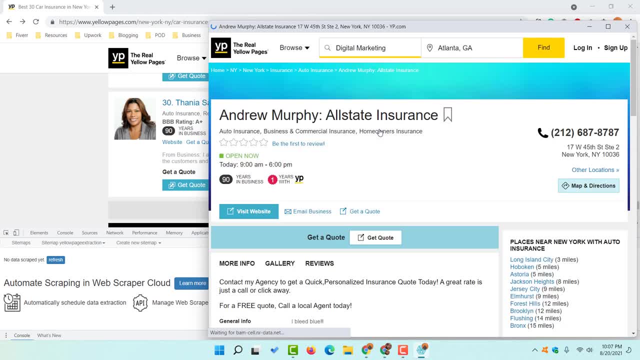 missing, or the phone number is missing, and this is because there are no information provided for these fields. and it happens because there are no information provided for these fields, and it happens for some pages. okay, so now, if i click on this refresh button, we are going to be able to see. 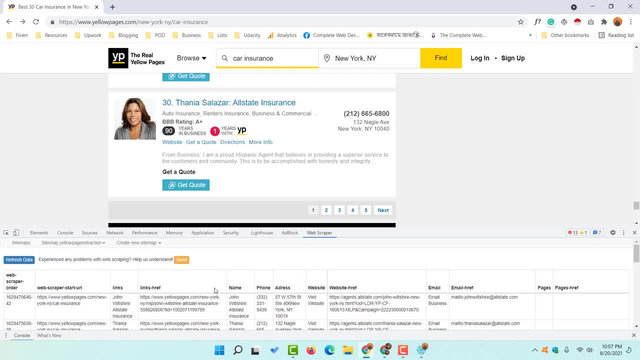 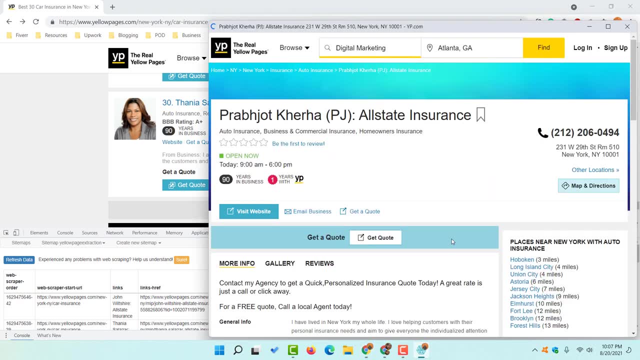 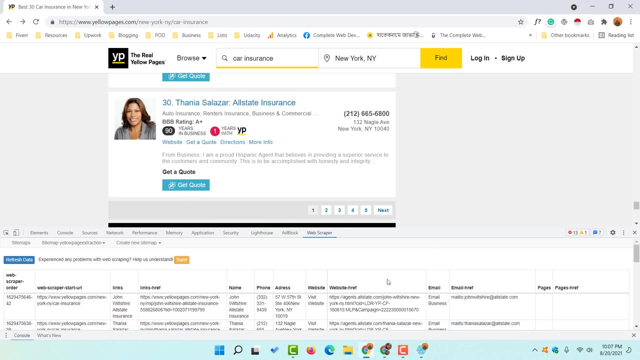 some information has been already populated here. just take a look now. the more time it will stay active in the background, the more data it is going to collect for us. so, as i have settled everything properly, it is going to visit each of these pages it is going to get the data from. 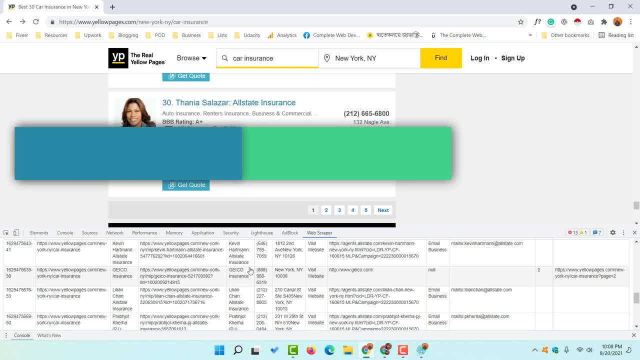 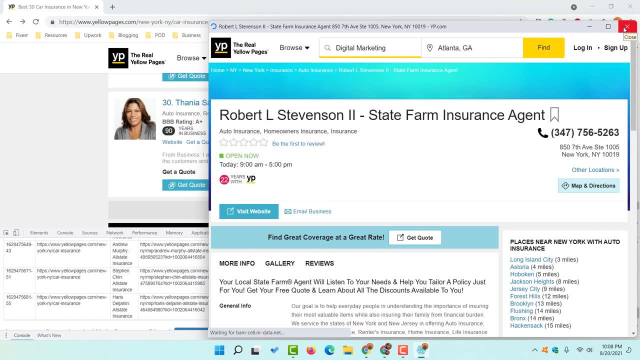 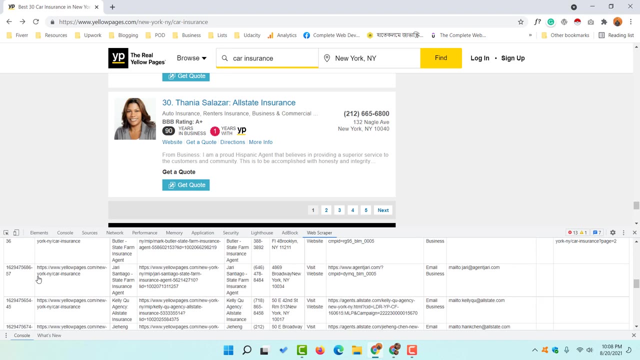 these pages automatically into our database. now it is going to do its work. so what i'm going to do, i'm going to close this data extraction process now and let me show you how much we have got as of now, these things. it's totally fine to show you the process of downloading your in results. so what i'm going to do, i'm going to 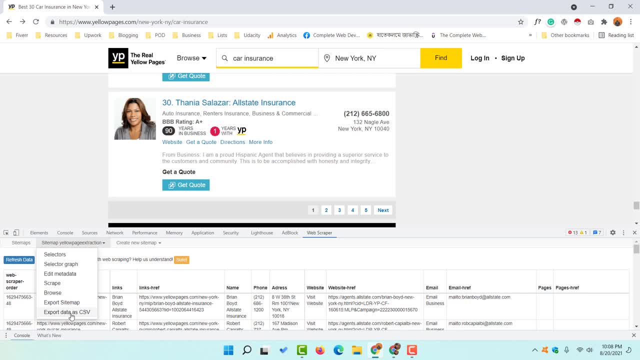 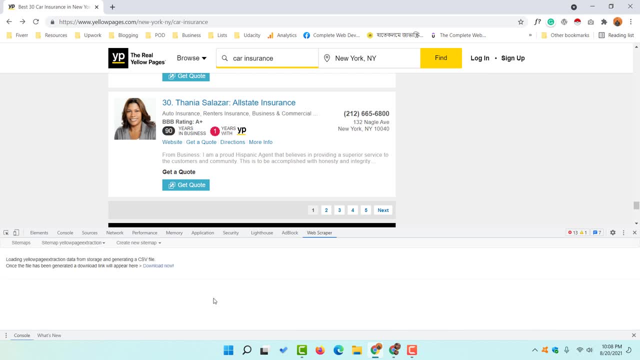 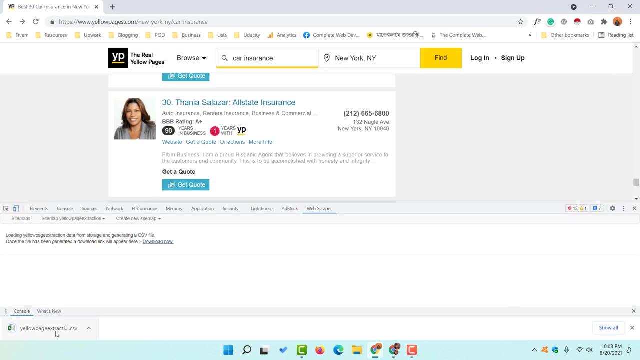 click on this button. after that you have to click on export data as csb to download it into your excel document. so let me click on it. after that, we're going to click on this download now button and then we have to click on save and the files will be saved on a csp file. now i'm going to open this file and, if you just notice, 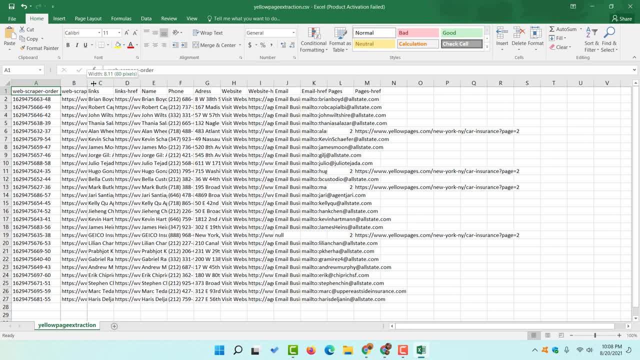 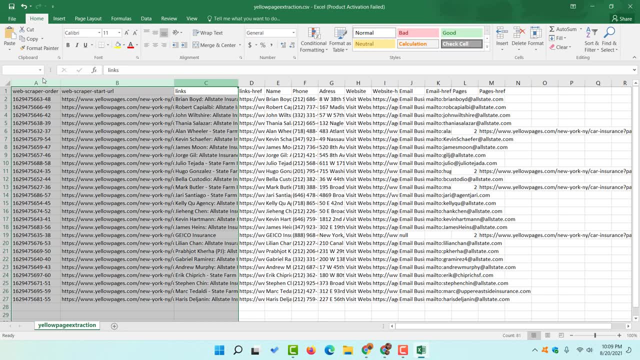 here we have got all the information. just take a look. all right, so now what i'm going to do. i'm going to clean this. um things up in real quick to show you the end result. i'm going to clean and i'd love to keep these. 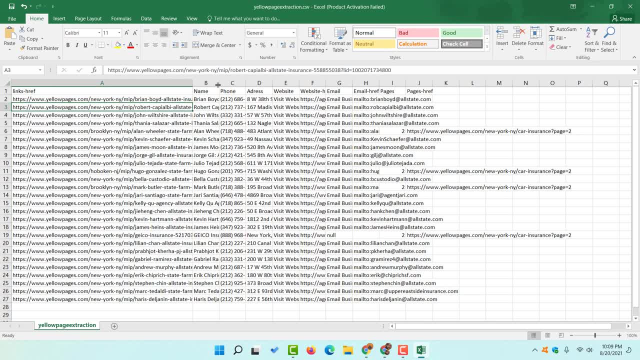 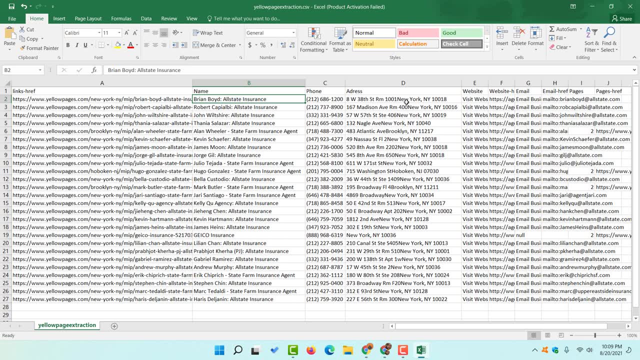 as a reference to each of these listings. then i have got this business or the person's name. we have got the phone number, address information, which includes the street address, city and state and the zip code. then i have got the website. i'm going to delete this one from here. 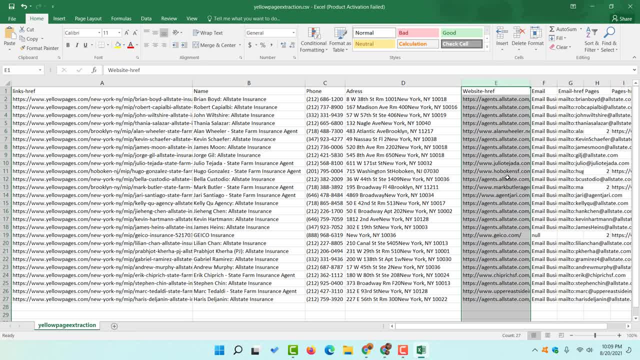 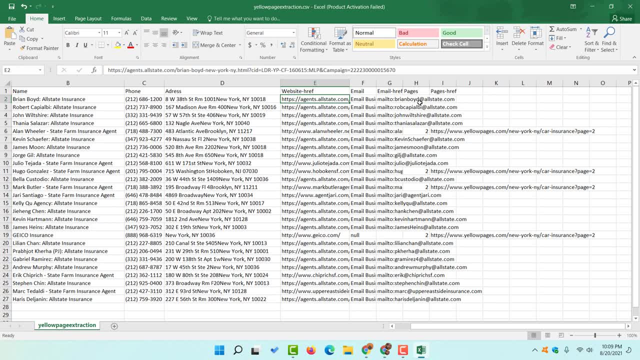 if you notice here we have got the website and, wow, it looks that we have got some uh, repetitive or let's say, duplicate websites. but i don't think these as duplicate because if you just notice here at these emails you want, you're going to see that these emails are different and the person names. 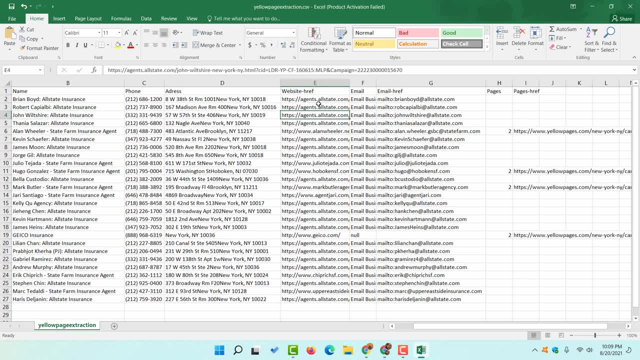 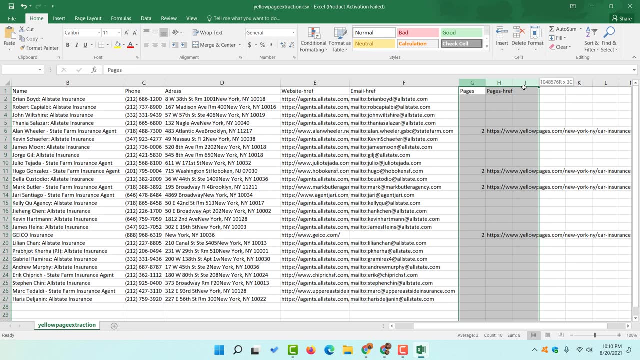 are different. so these are actually these businesses. uh has multiple people's listed on the listing, so this is the reason it. we are seeing some um relevancy here, so it is not a problem. then we have got this email field which we don't need. we don't need the other pages from here and 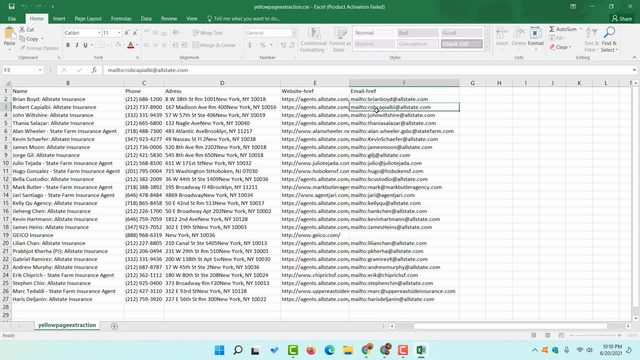 if you just notice here, we have got mail to these types of text appearing, you can see that we have got this email field which we don't need. we don't need the other pages on each of these emails. so what we can do, we can get rid of this easily. to do this, we have to 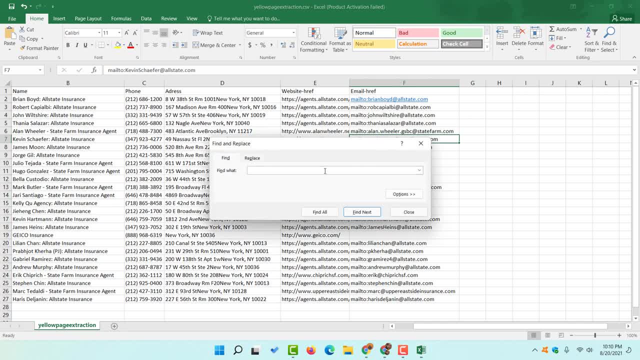 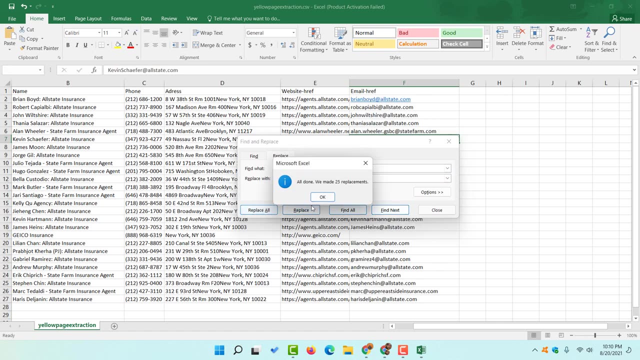 simply click on ctrl f into our keyboard and then you'll find this option: find and replace. then click on replace. we are going to type out this information like mail to mail to, and then this colon. then we're going to click on replace all and just take a look, we have got a clean. 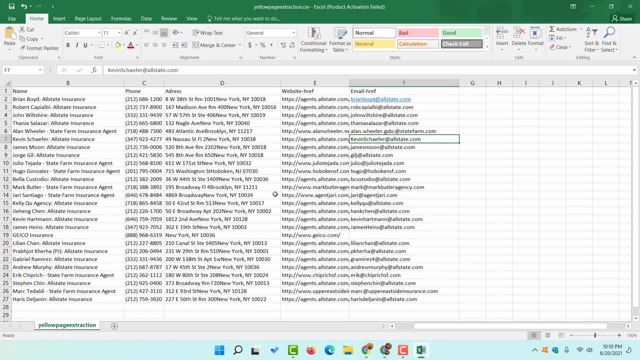 email list already, right, so we have got 27 listing. it's totally fine. so this was the process of automatically extracting data from any business listing website or any website. so i believe you have found this video helpful. if you did, please give this video a like, share this video to help your friends and let me know if you have any question. 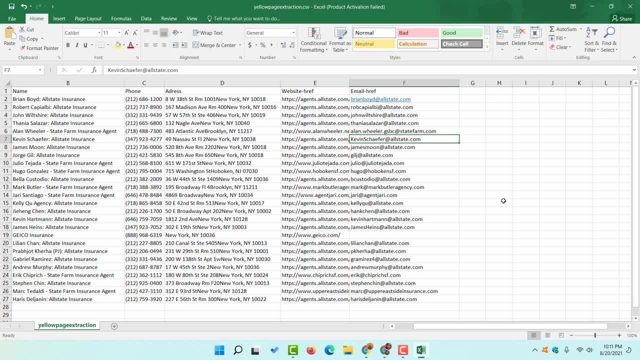 by commenting below and your opinion will be highly appreciated, and please subscribe to my channel to get more helpful videos in near future. i hope to see you in the next video. bye, bye, bye. see you in my next videos. have a good day, bye, bye. 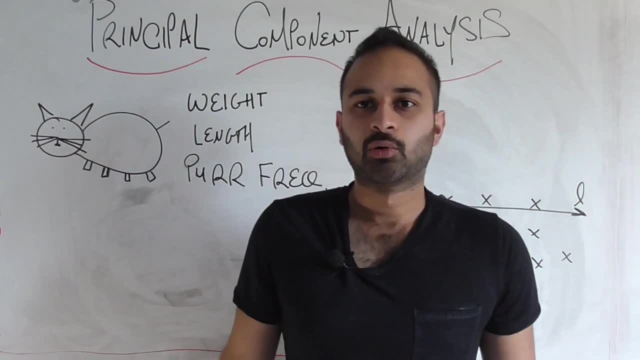 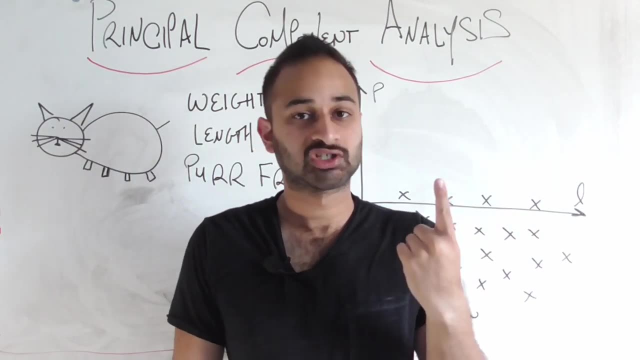 Hey, y'all how you doing. In this video we're finally going to get to talk about principal component analysis. So this is one of my favorite topics in data science for various reasons. One, just because it's so applicable and so useful in the real world. Second one is because it brings together so many of 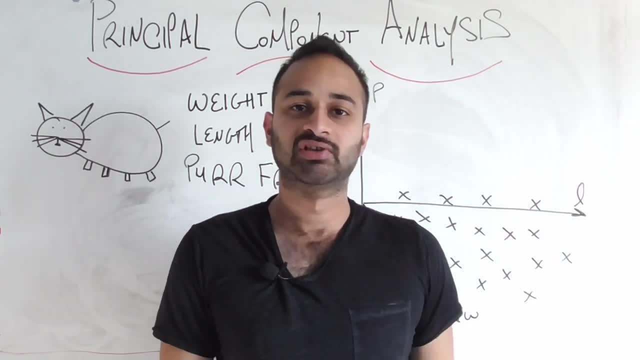 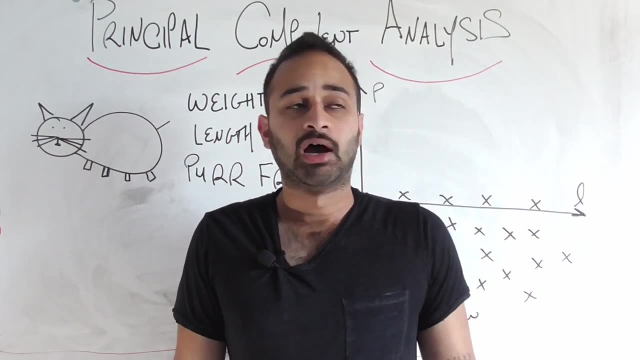 the mathematical foundations that we've been talking about building up in previous videos. Now we finally get to put them all to work in an actual data science machine learning context. Okay, I thought about how to structure the principal component videos. I think what I want to do is this video will be a 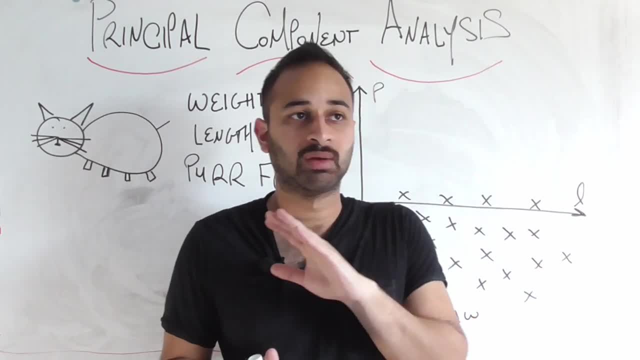 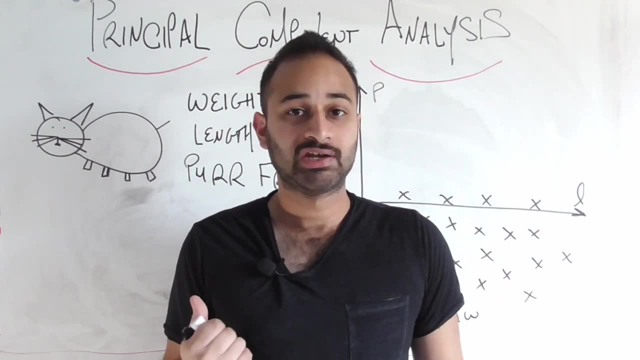 high-level explainer of principal component analysis. so don't worry about having watched any of the math theory videos, because we won't get into that in this particular video. We will get into that in the next video, which will be kind of a medium-level overview of what is principal component analysis. 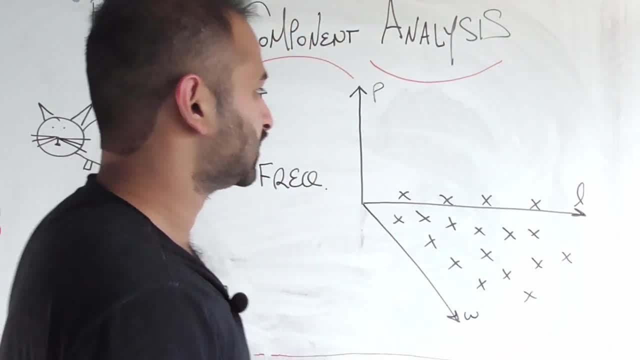 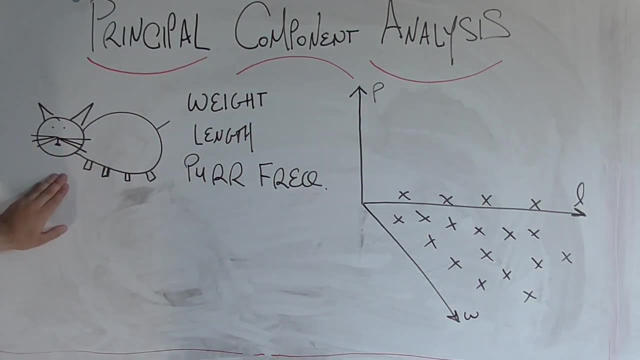 mathematically Okay. so let's get right into it. for this high-level explainer video, The context. as always, we're going to provide a context, so it's not just math. We have this beautiful camera. We have this beautiful camera. We have this beautiful camera. We have this.